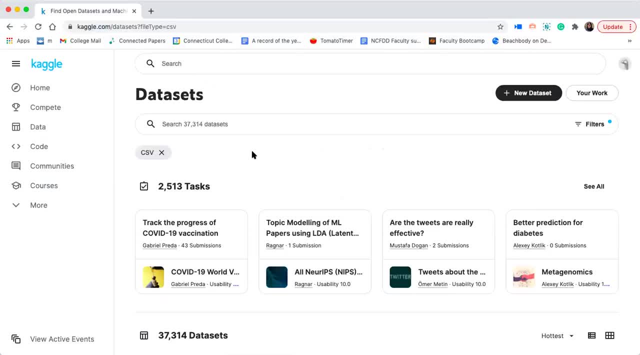 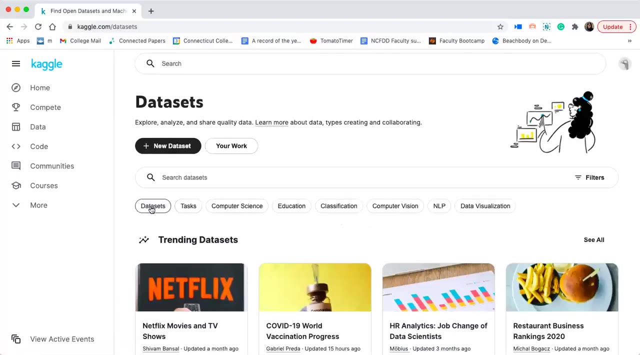 websites with you. so if you don't think you are going to find a data set from here, you may check other websites as well, And if you look at here it, you can see they have some keywords like datasets, tasks, computer science and so on. 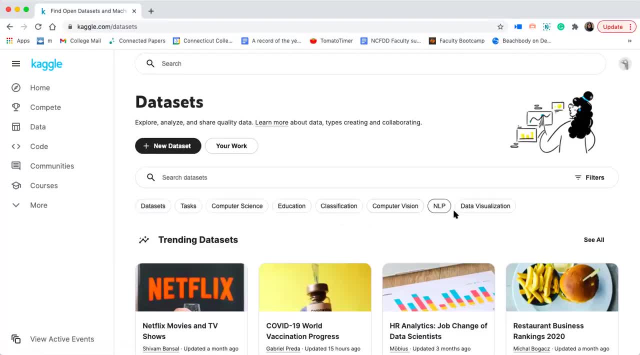 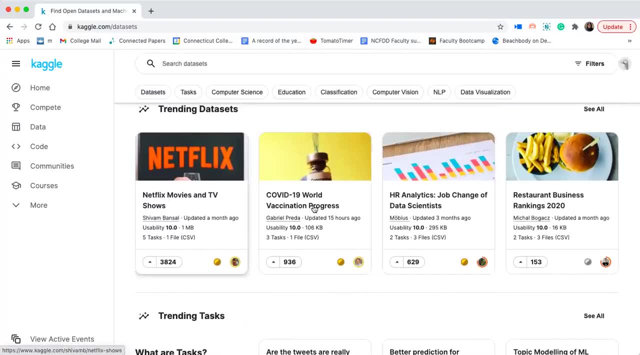 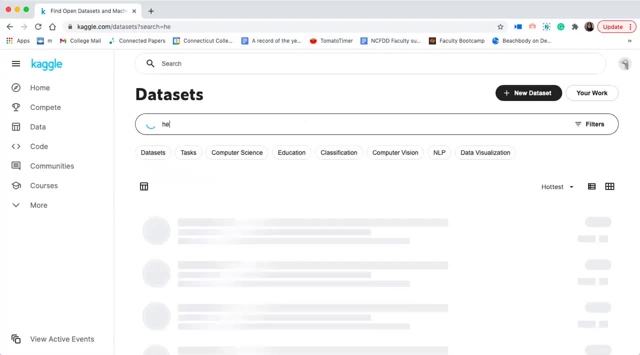 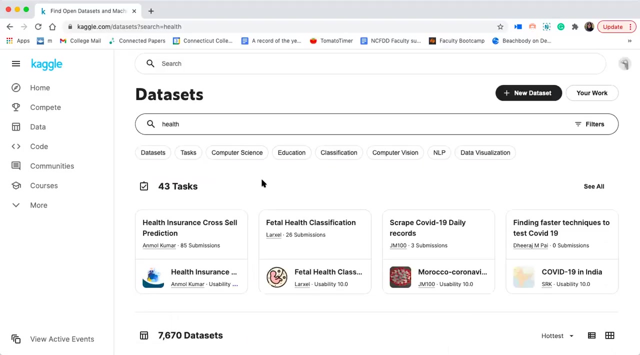 And they also have some trending datasets here. And also you can just do a quick search here. For example, if I want to work on health data, I may just type health and do a quick search on health. If you are interested in working on health data, you can type health and then click search and it will run to your data. 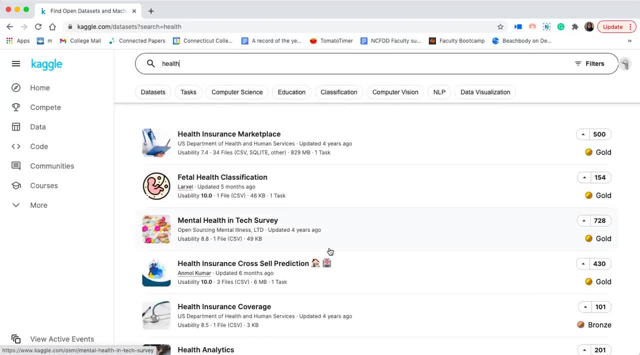 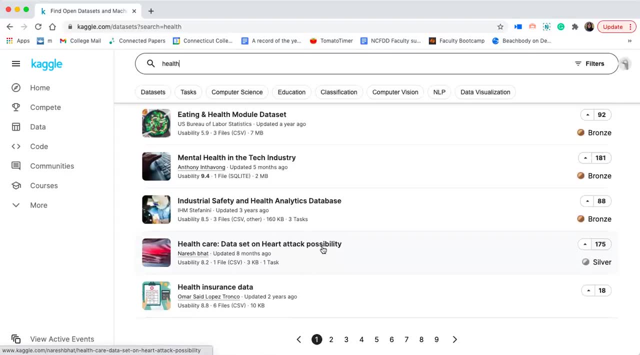 on health data. you may type the keyword there and you are seeing so many data sets here. i'm going to quickly pick a data set that may be of interest on me, for example, this one healthcare data set on heart attack probability. so i'm just going to click the title. 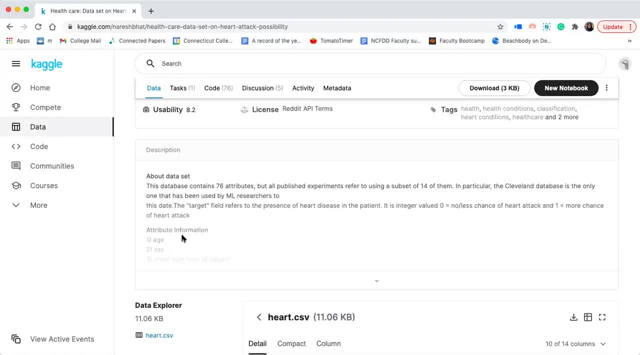 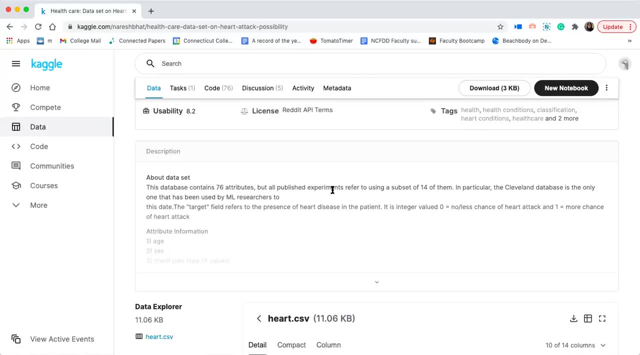 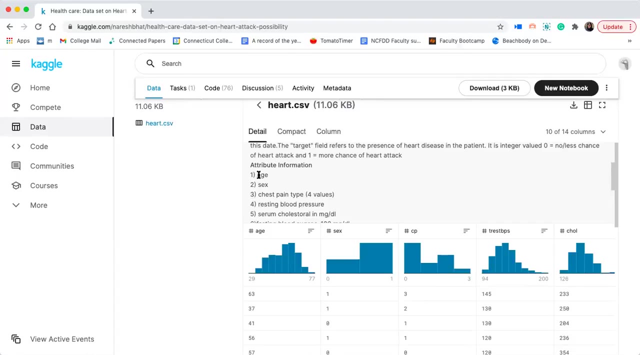 and here you are seeing a description of the data set. so about the data set: it has 76 attributes and and also all the details are here. so we have age, sex, chest pain type, including four values, and we have resting blood pressure and we have so many different. 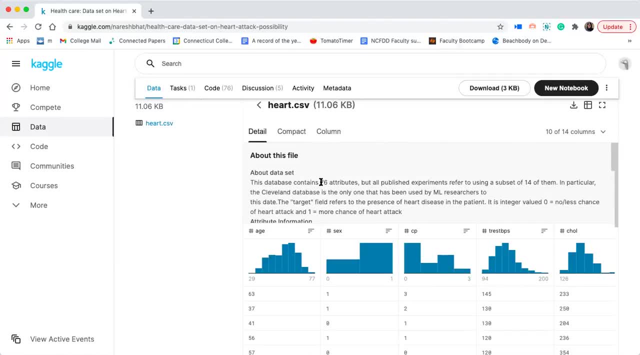 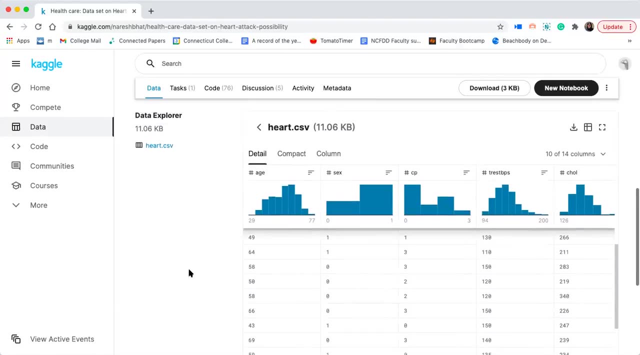 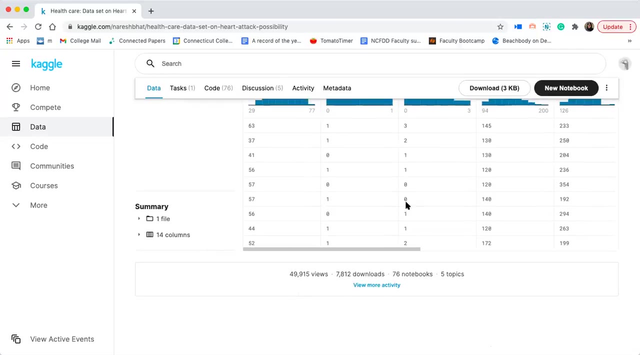 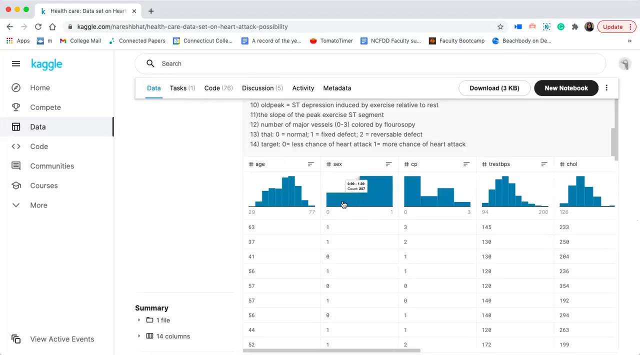 variables in this data, even though the um, let's say how many observations we have. i don't think they mentioned it, but take a quick look at the data you are seeing. we have like, for example, the age variable is roughly normally distributed and the sex variable is just zero and one. so, looking at this data you are seeing 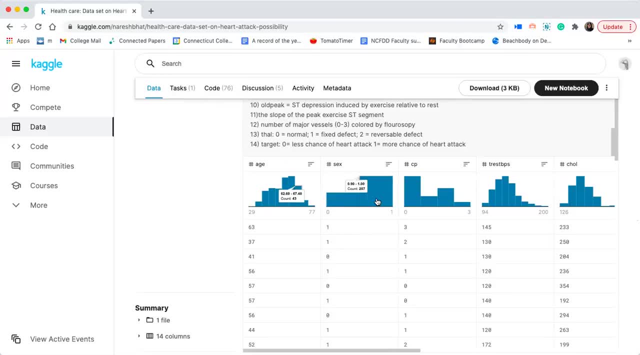 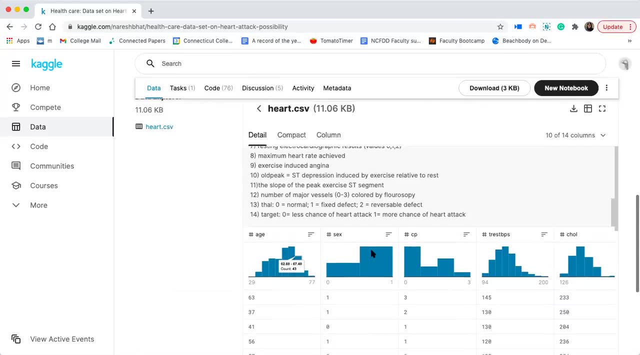 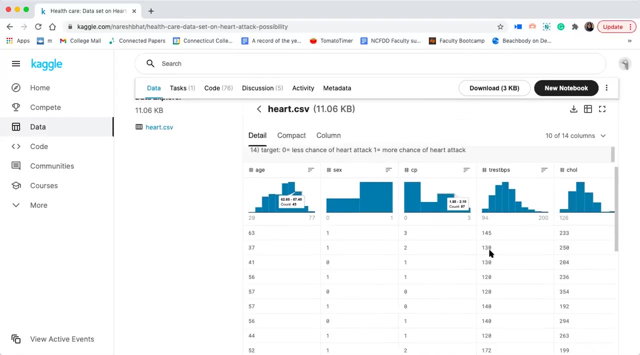 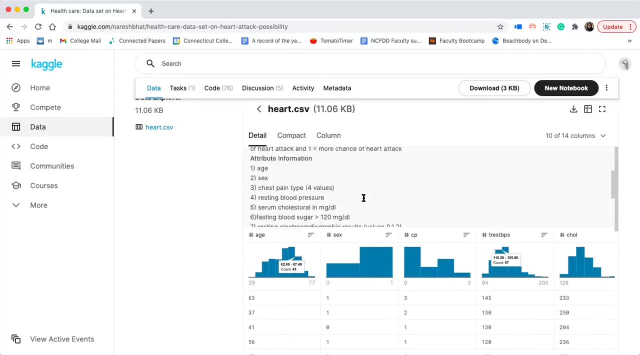 they have 96 zeros and 207 ones. that means that this data has at least 300 observations, which is which will be a good data set for a class project, and they even have like a cluster level. they have. they have a few categorical variables and a few um numerical variables as well. 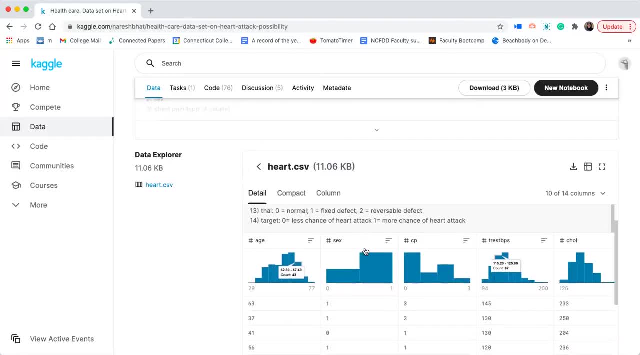 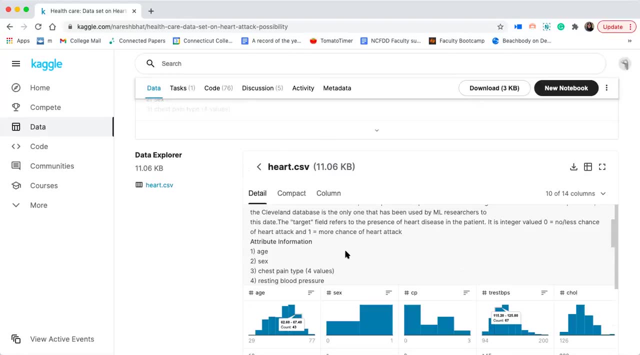 so in a class project, as in the regression models class. that's what we want. we do really need categorical variables and we want numerical variables so that you can actually propose several different questions and especially the questions can be answered using, like a simple linear regression model, multiple linear regression model. 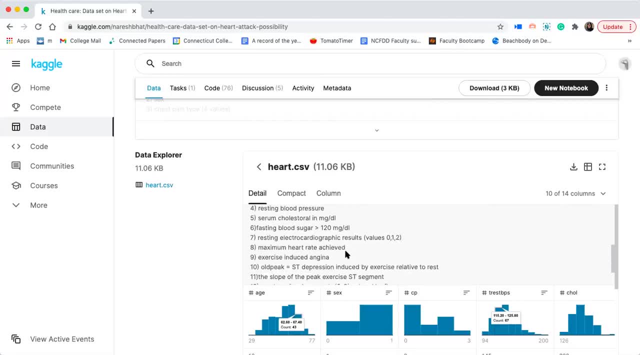 anova and logistic regression. so you can see here they have: the target variable is less chance of heart attack and the one is more chance of a heart attack. so this variable, target, is a binary variable which only has zero and one values. so if you ask a question, 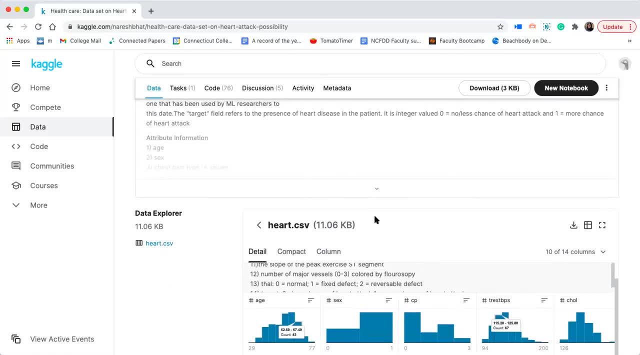 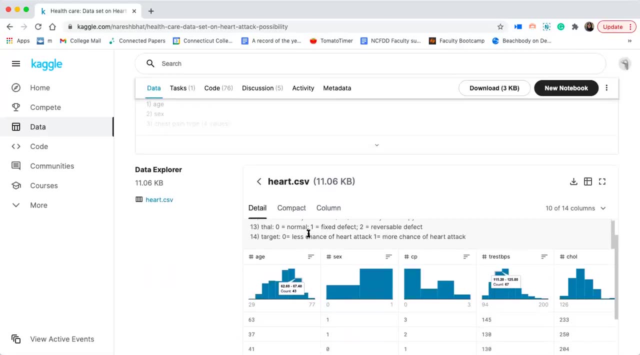 what are the factors in the analysis? factors that is, affecting the probability or the likelihood of getting heart disease. So the response variable will be the target variable, which is a 0, 1 variable, And the predictors will be the variables from the other 13 variables. 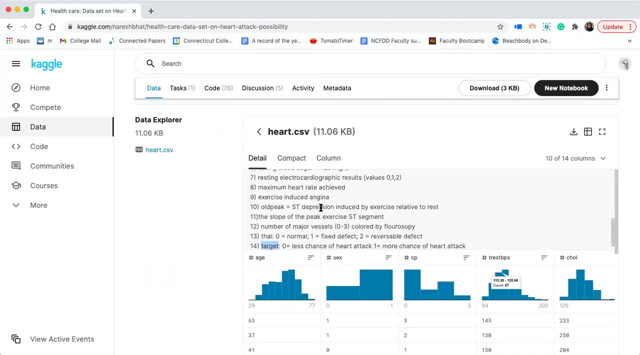 So it can be any of the combinations after you explore different kinds of models, But that will be a question to be answered using logistic regression. So that is the last model we are going to talk about in the class, And maybe you can also ask a question like: is there a difference in the cholesterol level? 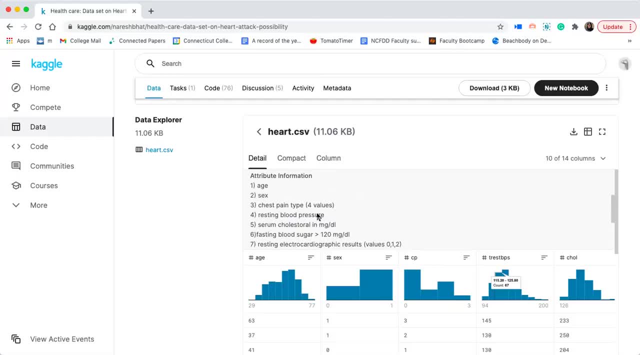 of different chest pain type. So the response variable is numeric And the Predictor is actually a categorical variable including four categories. So that is a question can be answered by using ANOVA models, And you can come up with other interesting questions as well. 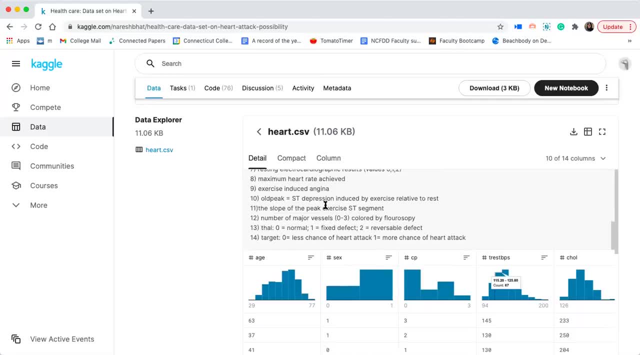 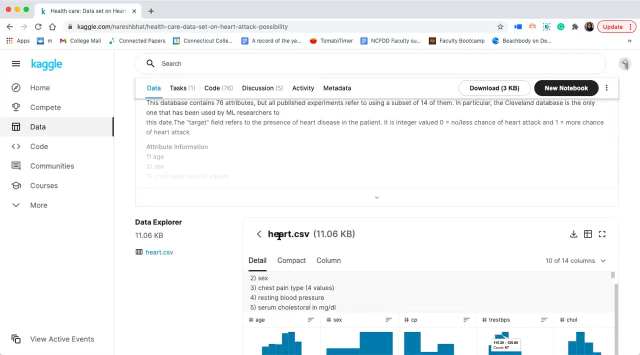 But I'm just showing you some examples where you may ask meaningful questions And also those questions can be solved and can be answered using the data that you have here And you can see this data set is heartcsv. You can actually click here to download the data. 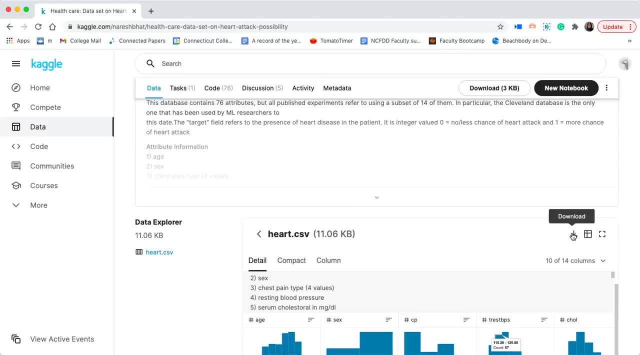 So after you download the data, you know how to import it into RStudio And then you can do data management, data visualization and do the modeling in RStudio, Just to use what you have learned during the semester. So I can click download. 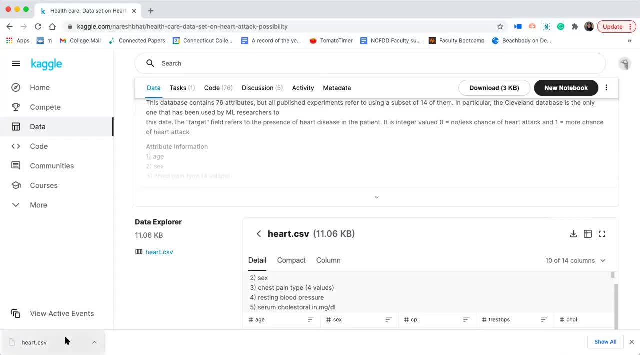 And you can see the heart data set is downloaded So I can actually click to open it to have a quick look at it, or you can just import it into RStudio. So once I click open to view the data, I'm not going to save it. 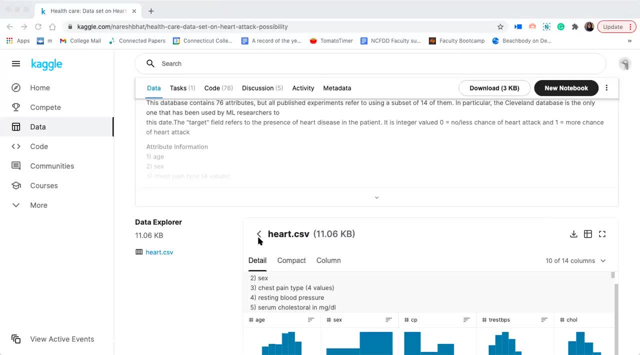 I'm not going to do anything because I want to keep it to be the CSV file. So when I import, When I imported the data set into RStudio, I will not save it. I will not have a problem. So this is the data. 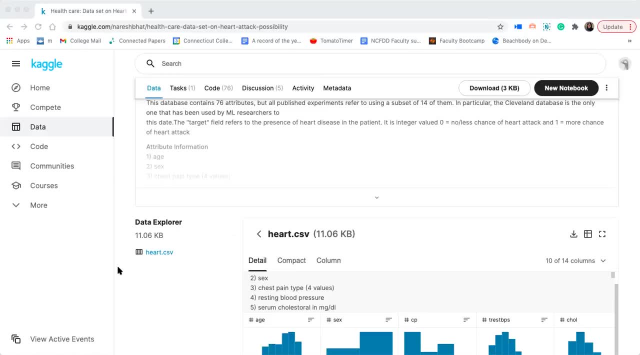 You can see you have. You have a long list of observations, So, which is great. You don't want to have only 10 or 20 or just 50 observations for class project And that's it. So, once you have the data based on the variables, what kind of questions you want to explore? 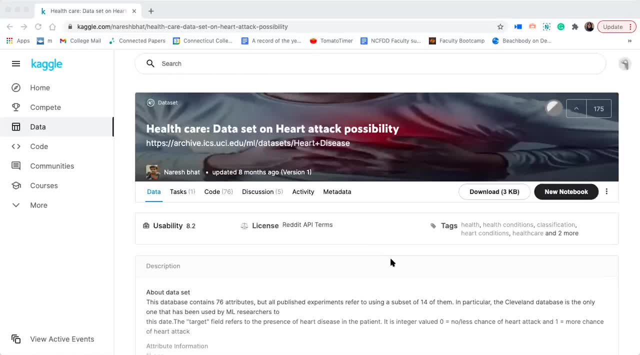 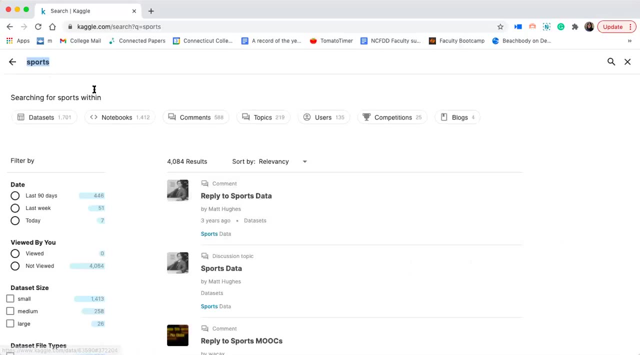 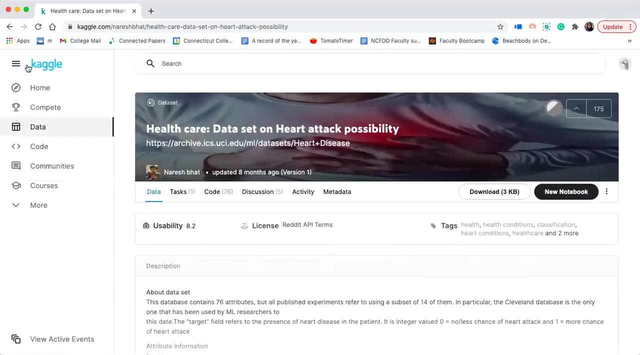 you just bring up the questions And then try to find the best model to answer those questions. And again, you can actually do some sparse analysis as well, Like just based on your interest. you can. you can even search sparse. I'm going to go to the data sets page.